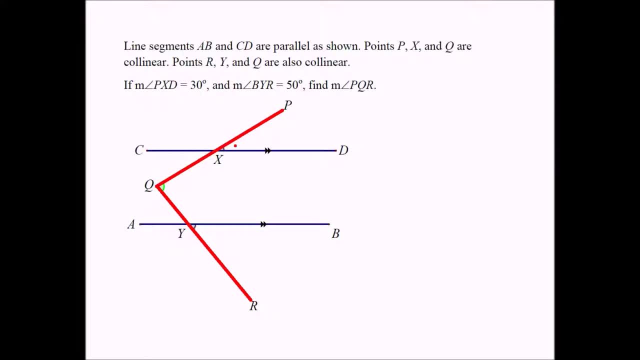 We know this angle. This is PXD, which is a straight line. We know that this angle is 30 degrees and this angle is BYR, which is 50 degrees, And we are supposed to find this angle. How do we do that? 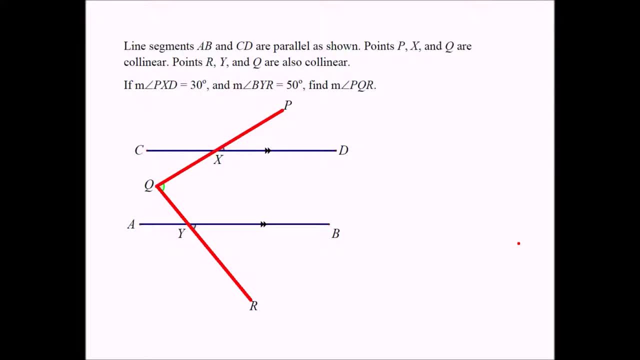 So go ahead, Try to solve the problem on your own. See if you can solve it. If you cannot, please follow the video that follows. So let's go ahead and label a few things. This is 30 degrees And this is. 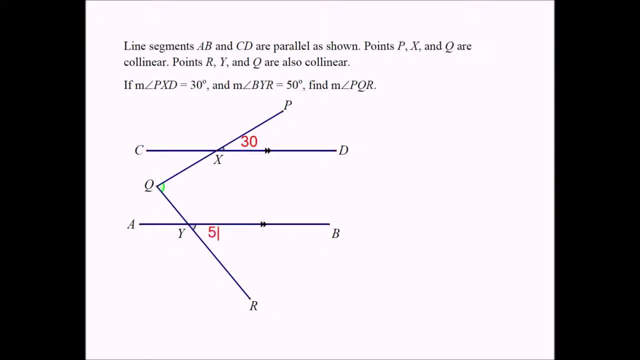 50 degrees Now. in geometry we cannot change the figure that's given to us, but we can add things to the figure. So let's go ahead and draw a line through the point Q that is parallel to the line segment AB, and that's how we're going to. 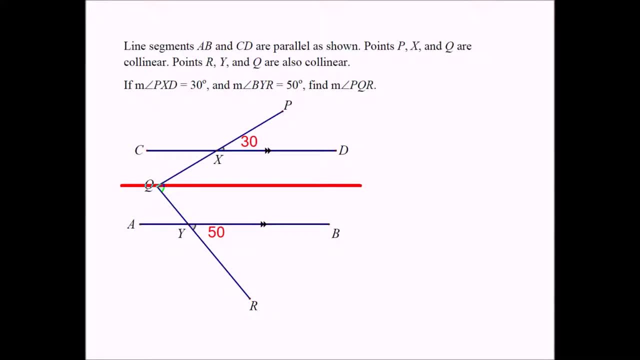 do it. So we are constructing this red line which is passing through the point Q, and it is constructed in a manner so that this red line is parallel to the line AB. I'm going to mark it with double arrows, just like the other two lines are marked Now, if the red line is parallel to AB, since AB is parallel to CD. 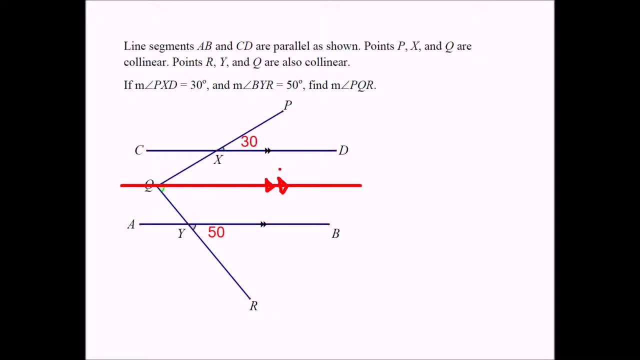 the red line must be parallel to CD. Now this angle has to be 30 degrees because these are corresponding angles and these two lines are parallel. So I'm going to write 30 degrees. I'm going to use a different color here: 30. These two angles are corresponding angles and these two lines. 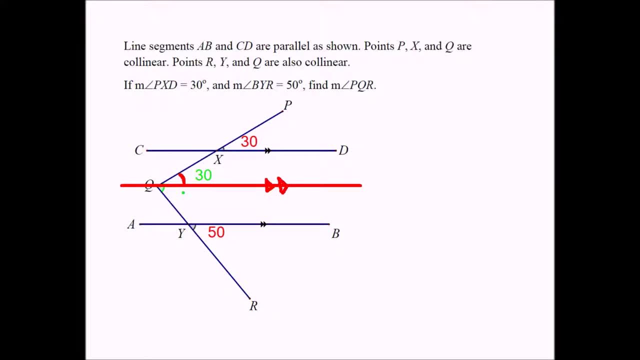 are parallel, so this should also be 50 degrees, Therefore angle PQR. therefore, angle PQR must equal 30 plus 50, equal to 80 degrees. That's my answer: 80 degrees. Thank you.